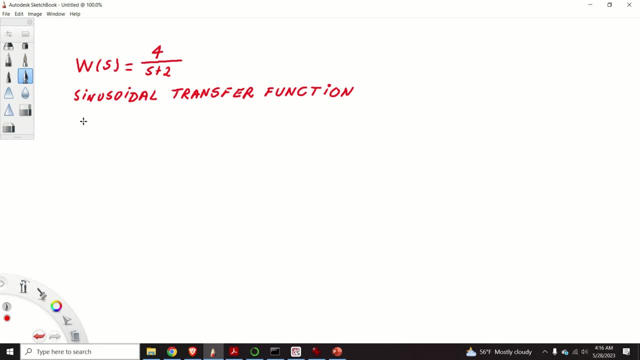 The first step is to derive the sinusoidal transfer function. We obtain the sinusoidal transfer function by substituting s by j, omega in our transfer function. Here j is the imaginary unit, That is, it's equal to square root of minus 1, and omega is the angular frequency. 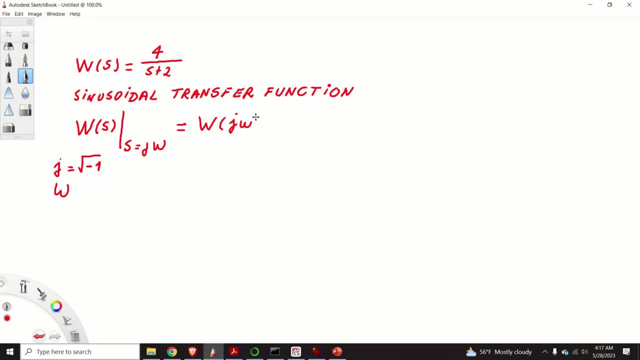 After we substitute s by j omega, we obtain this expression: 4 over 2 plus j omega. Obviously, this transfer function is a complex number that depends on omega. Every complex number has a real part and an imaginary part, And it can be represented as a point in a complex plane, with its real part and with its imaginary part. 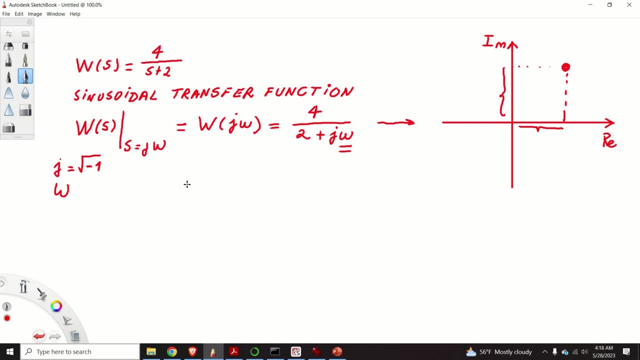 Our next task is to compute the sinusoidal transfer function. It is to compute the real and imaginary parts of this transfer function. What is the easiest way to do that? The easiest way to do that is to multiply the numerator and the denominator of our original transfer function. 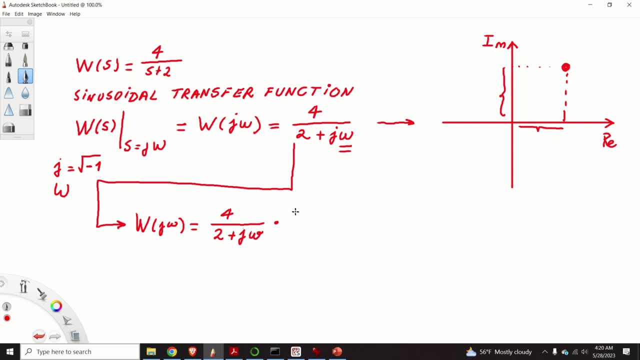 or better to say, sinusoidal transfer function by 2 minus j omega over 2 minus j omega. Obviously, 2 minus j omega over 2 minus j omega is equal to 1, and nothing changes, However, by multiplying the denominator by 2 minus j omega. 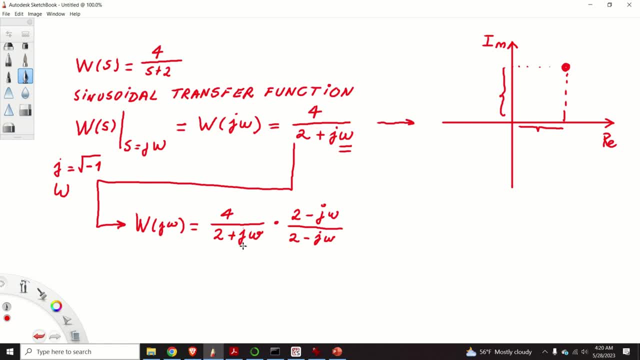 we will get rid of the complex number in the denominator. Consequently, we obtain the following expression In the numerator: we have 4.. Multiplying 2 minus j, omega, In the denominator we have the following expression: 4 plus omega, square. 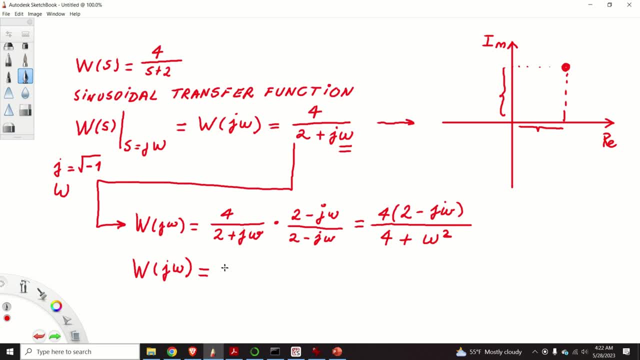 Consequently, our sinusoidal transfer function can be written as follows: 8 over 4 plus omega square minus 4. omega over 4 plus omega square multiplying j. From this expression we can observe that the real part of our sinusoidal transfer function. 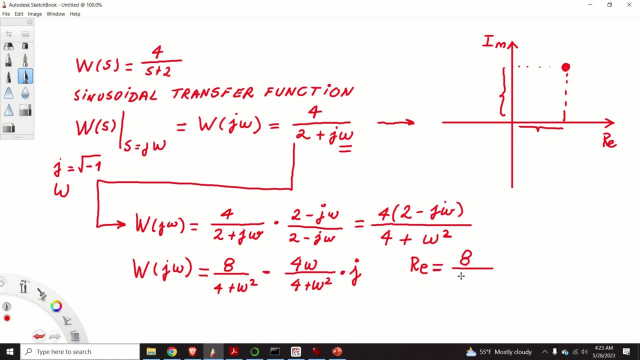 is equal to 8 over 4 plus omega square. The imaginary part, on the other hand, is equal to minus 4 omega over 4 plus omega square. These expressions are necessary for sketching the Nyquist plot by hand, The Nyquist plot of the transfer function w of j omega. 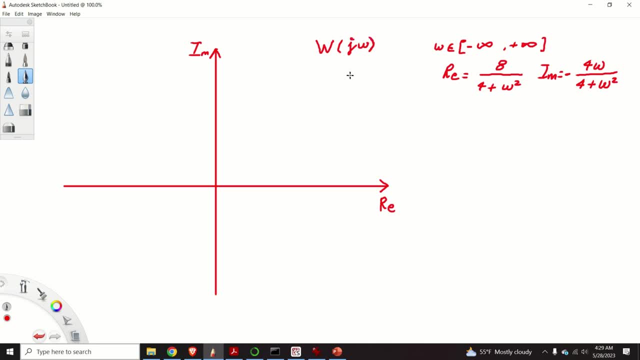 is a path in the complex plane that the sinusoidal transfer function describes, or, better to say, the path that this complex number describes when omega is varied from minus infinity to plus infinity. In practice, we only vary omega from 0 to plus infinity. 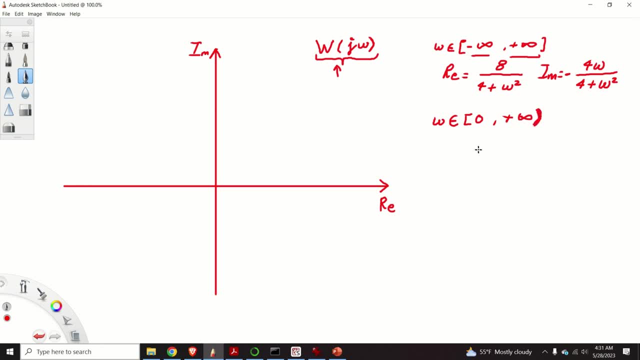 And we sketch the part of the Nyquist plot corresponding to these values of omega. The other part of the Nyquist plot is simply obtained by mirroring the first part of the Nyquist plot with respect to the real axis. To sketch the Nyquist plot, we will construct this table. 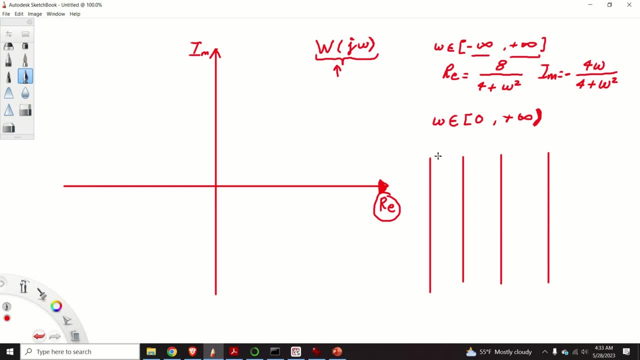 The first column of this table corresponds to characteristic values of omega. The second column corresponds to the real part of sinusoidal transfer function and the third column corresponds to the imaginary parts of the transfer function. Let us start from 0.. When omega is 0,, the real part is obviously equal to 2.. 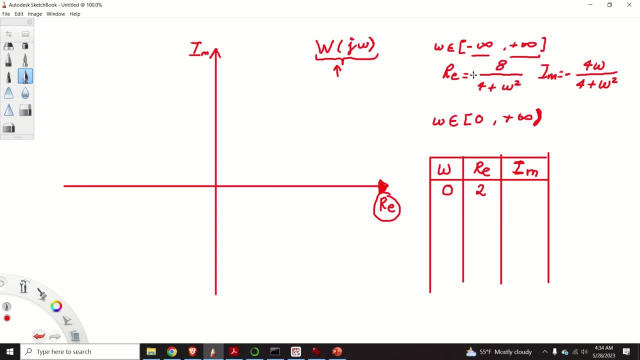 You can obtain this real part by substituting 2 for omega. in this expression, The imaginary part is equal to 0. Consequently, our plot starts from this point on the real axis And over here. it is always a good practice to change the color. 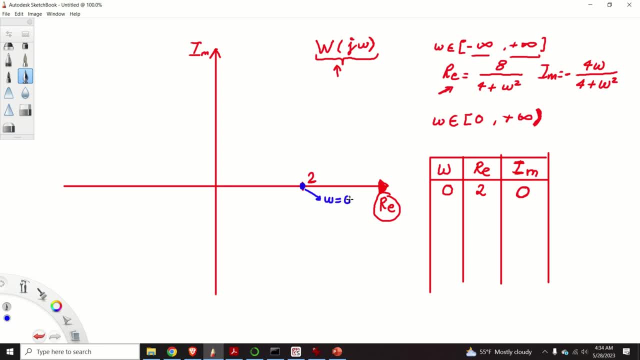 and to specify the value of omega, Omega is equal to 0.. The second characteristic point can be, for example, that omega is equal to 1.. When omega is equal to 1,, the real part is equal to 8 over 5. 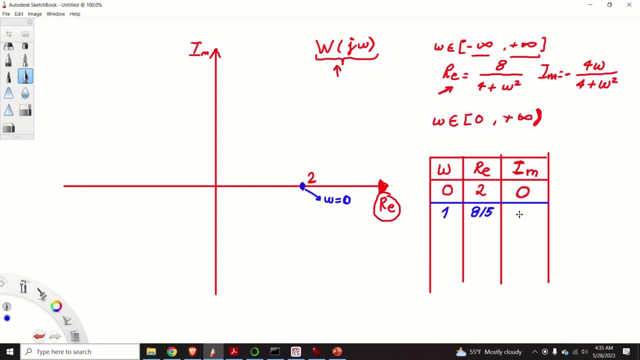 and the imaginary part is equal to minus 4 over 5.. 8 over 5 is equal to minus, 8 over 5 is equal to 8 over 5 and minus 4 over 5 correspond to a point somewhere over here. 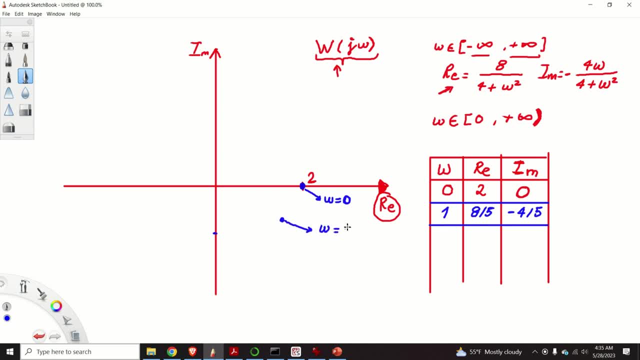 This point is obtained for omega is equal to 1.. The next characteristic frequency is: omega is equal to 2.. For omega equals to 2, obviously the real part becomes 1 and the imaginary part becomes minus 1.. The point 1 and minus 1 is this point over here. 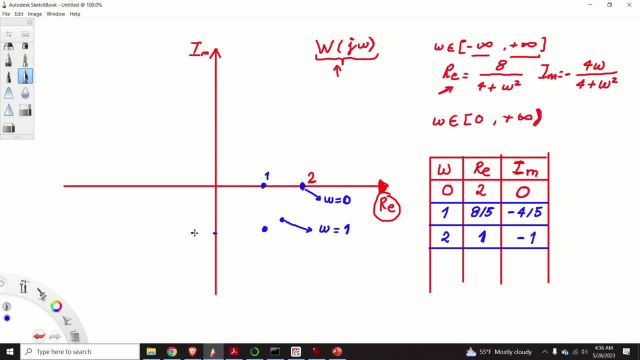 This is 1 and this is minus 1.. And this point is obtained, for omega is equal to 2.. Another characteristic point is obtained, for omega is equal to 4.. For omega is equal to 4, we have that the real part is actually 2 over 5. 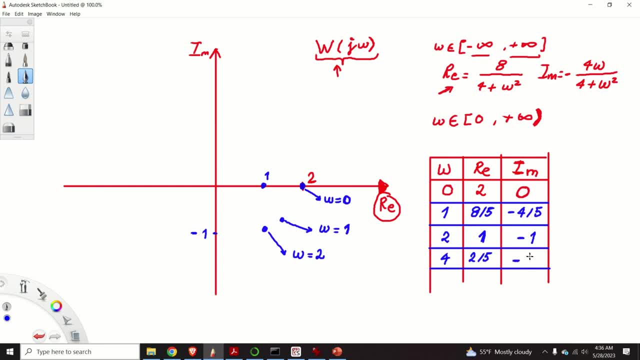 and the imaginary part is actually 2 over 5.. And the imaginary part is actually 2 over 5.. And the imaginary part is equal to minus 4 over 5.. This point is the point over here, And this point is obtained, for omega is equal to 4.. 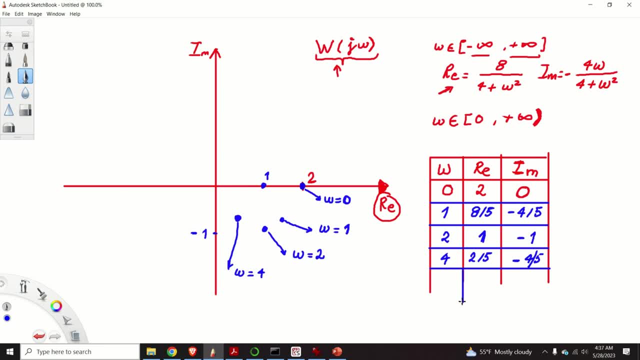 You can also construct other points by varying omega. You can take some other characteristic points. For example, omega is equal to 5,, 10,, 15, etc. However, We can clearly observe that as omega increases, the real part decreases and the imaginary part increases. 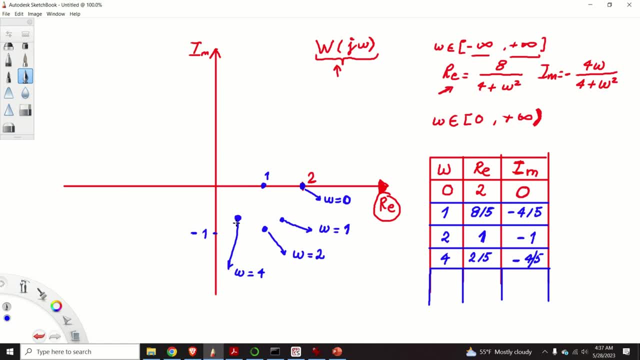 Imaginary part is negative, so its absolute value actually decreases. The final characteristic point is infinity point. That is, that's the point for which omega is equal to infinity. When omega is equal to infinity, the point is negative. When omega is equal to infinity, the point is negative. 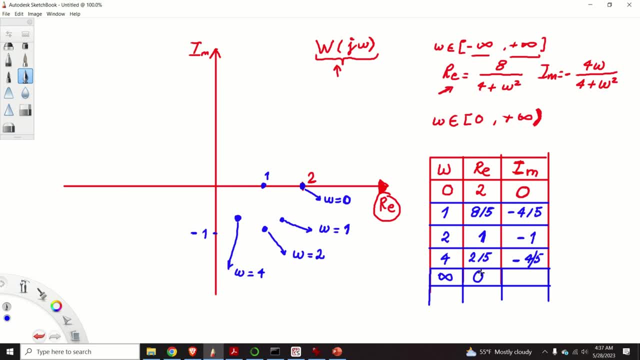 When omega is equal to infinity, the point is negative. Obviously, the real part becomes 0. And the imaginary part becomes a small negative number. When I say a small negative number, I mean a negative number that has a small absolute value. 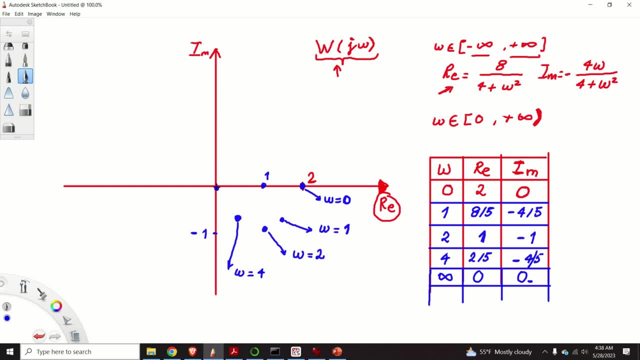 And, consequently, this is the point obtained, for omega is equal to infinity and, consequently, this is the point obtained, for omega is equal to infinity. The final step is to connect these points, and I will use green color to connect these points. So this is our first part of the Nyquist plot. The second part, obtained when 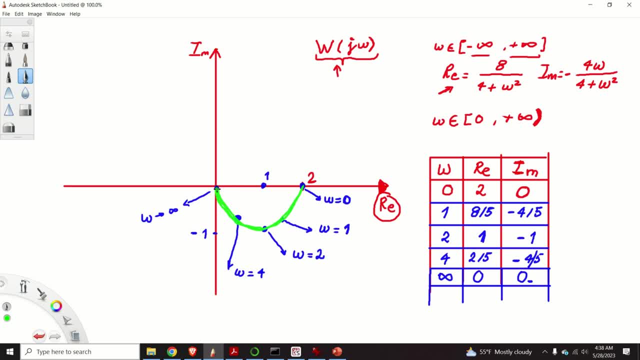 omega is from minus infinity to 0, is simply obtained by mirroring the first part. Here I'm trying to mirror the first part, and this is the final form of our Nyquist plot. Here we go from 0 to plus infinity and over here. 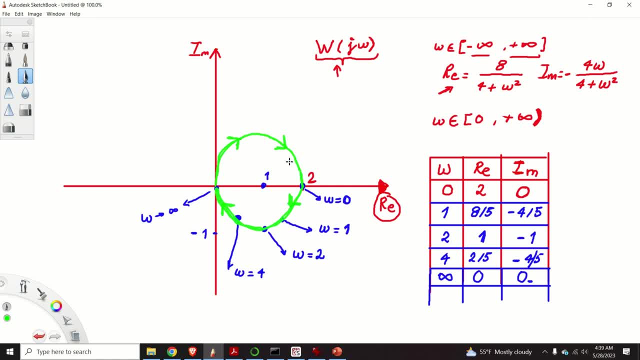 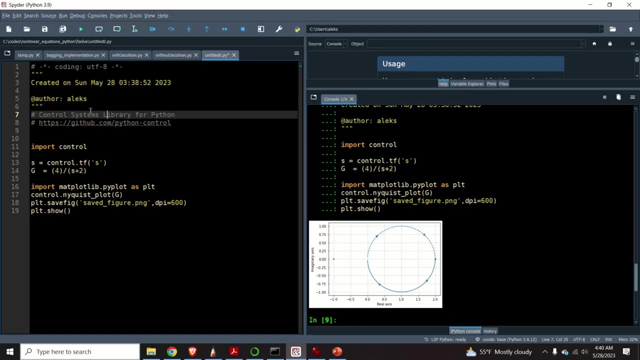 we go from minus infinity to zero. okay, so that was our Nyquist plot. next let us see how to precisely draw this plot in Python. as I mentioned at the beginning of this video, I'm using using the control systems library for Python. this is an open source and free library for control system design, analysis and this.